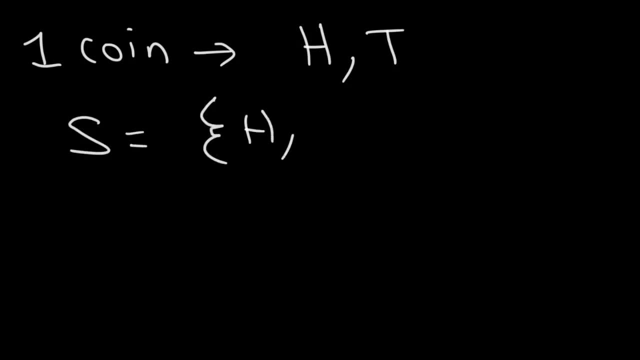 situation is either heads or tails. Now what if we wanted to flip, let's say, two coins? What are the possible outcomes? What's the sample space for flipping two coins? To help us get the answer, we're going to create something known as a tree diagram. So when flipping the first, 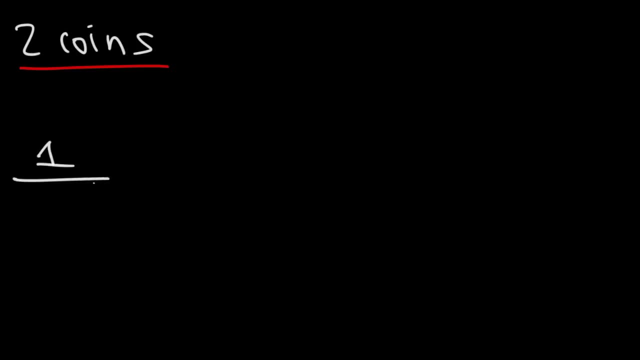 coin we have two possibilities: heads or tails. Now let's say, if we get heads for during the first flip, During the second flip we can get another two possibilities: heads or tails. Likewise, if we get a tails during the first flip, on the second flip we can also get heads or tails. So notice that we have four. 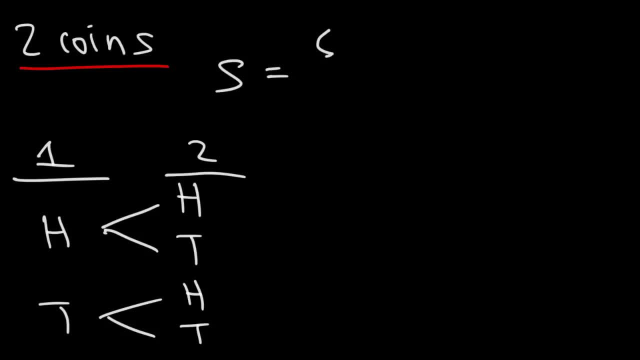 possible outcomes. So the sample space is going to be the first outcome, which is heads and then heads, so we can write that as HH. The second outcome is heads and then tails, so that's going to be HT. The third outcome is tails then heads. 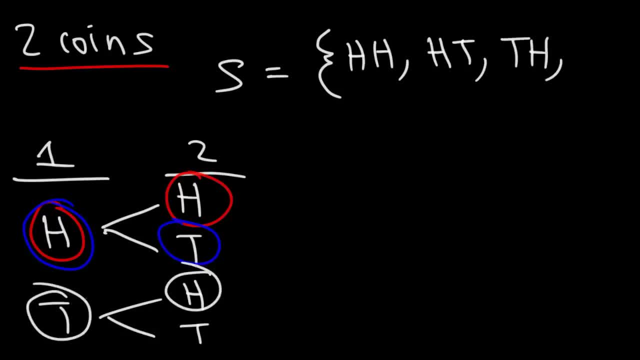 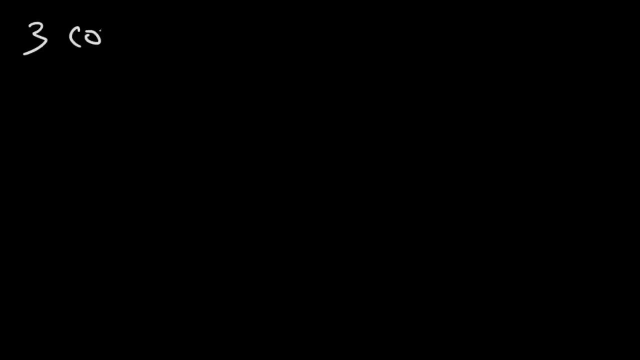 and the fourth outcome is going to be tails and then tails. So this would be the sample space of flipping two coins. Now, for the sake of practice, what is the sample space of flipping three coins? Feel free to pause the video and try that Construct the tree diagram to help you do so. So on the first try, we 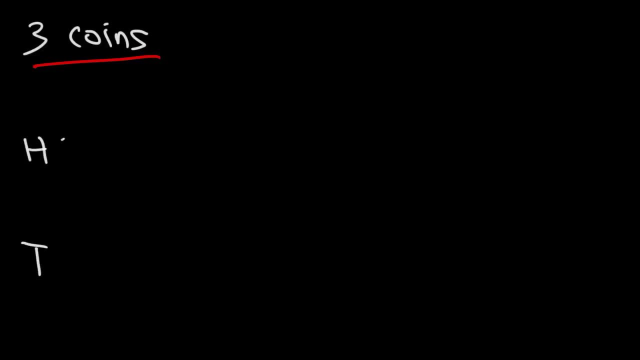 can get heads or tails. Now, if we get heads, it can be heads or tails, and if we get tails, it can also be heads or tails. Now, because we're flipping three coins, you need to do this one more time, So this could be H or T and then repeat the. 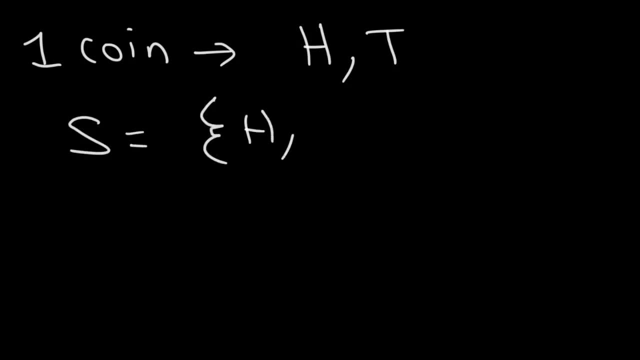 situation is either heads or tails. Now what if we wanted to flip, let's say, two coins? What are the possible outcomes? What's the sample space for flipping two coins? To help us get the answer, we're going to create something known as a tree diagram. So when flipping the first, 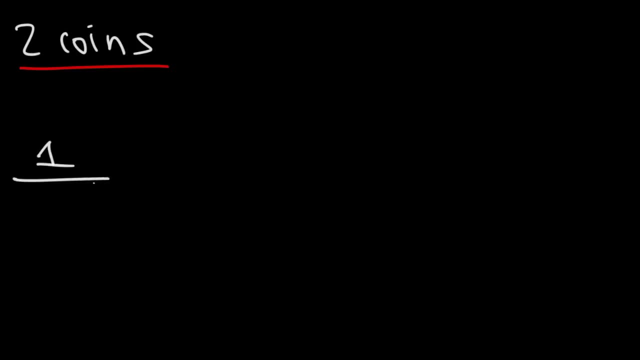 coin we have two possibilities: Heads or tails. Now let's say, if we get heads during the first flip, During the second flip we can get another two possibilities: heads or tails. Likewise, if we get a tails during the first flip, on the second flip we can also get heads or tails. So notice that we have four. 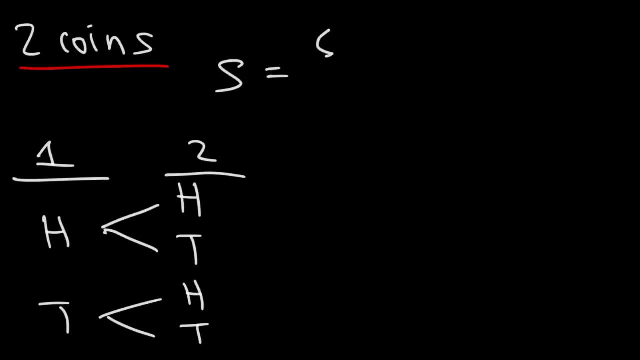 possible outcomes. So the sample space is going to be the first outcome, which is heads and then heads, so we can write that as HH. The second outcome is heads and then tails, so that's going to be HT. The third outcome is tails then heads. 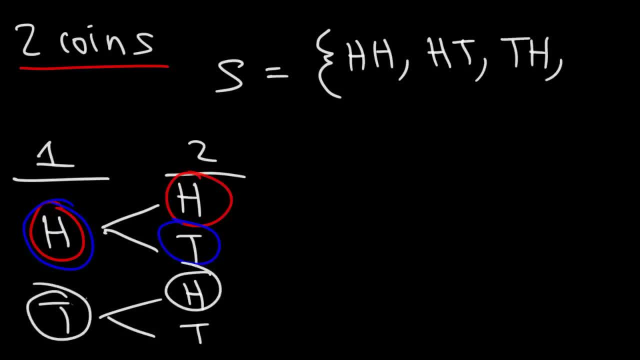 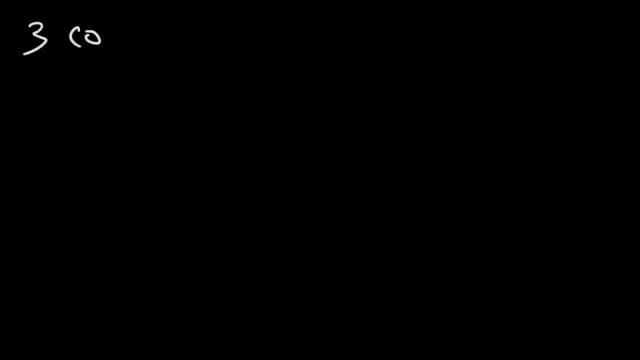 and the fourth outcome is going to be tails and then tails. So this would be the sample space of flipping two coins. Now, for the sake of practice, what is the sample space of flipping three coins? Feel free to pause the video and try that Construct the tree diagram to help you do so. So on the first try, we 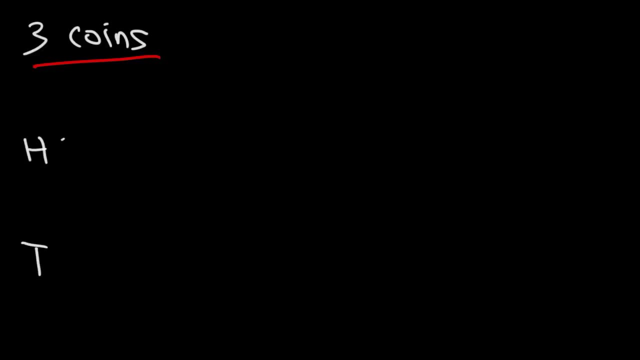 can get heads or tails. Now, if we get heads, it can be heads or tails, and if we get tails, it can also be heads or tails. Now, because we're flipping three coins, you need to do this one more time, So this could be H or T and then repeat the. 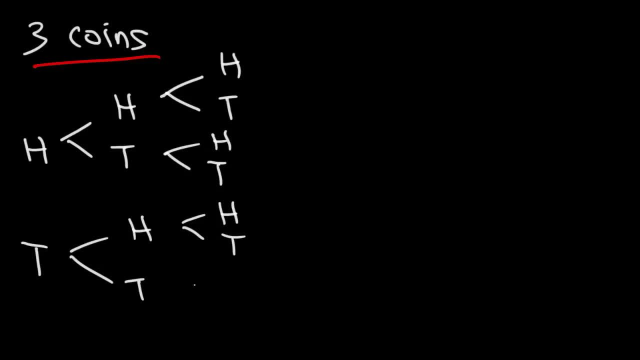 process For each one. So here's the first possibility: We can get three heads, So I'm going to write that as HHH. The second possibility is getting heads, heads and then tails, So HHT. The third possibility is: heads, tails, heads, So that's HTH. The fourth is: 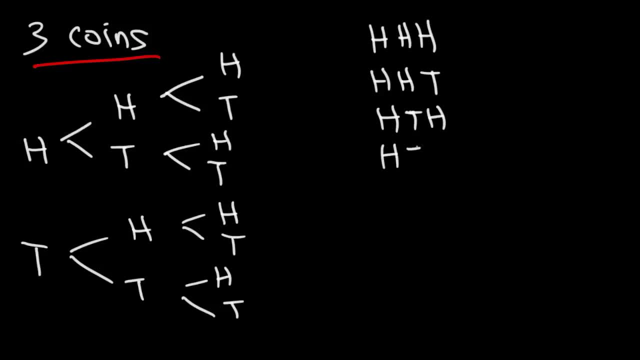 heads, tails, tails, So HTT, and then repeat. in this process, We see that the next one is going to be THH and then THT, TTH, and the last one is going to be TTT. So we're flipping two coins three times. 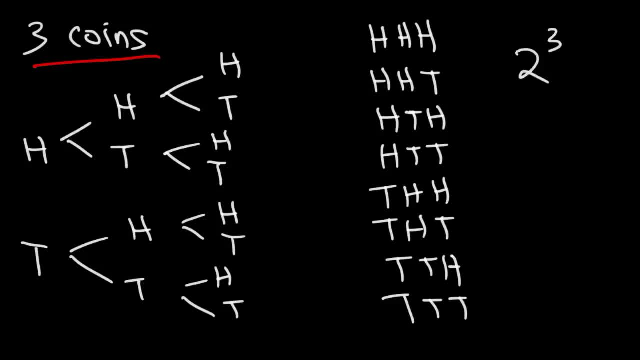 So the number of possible outcomes is 2, raised to the third power, which is 2 times 2 times 2, and so it gives us eight possible outcomes. So this is the sample space, which represents all the possible outcomes that we can get for flipping. 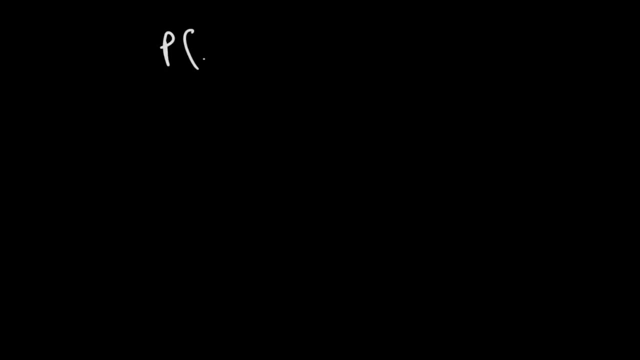 three coins. Now, the probability of an event occurring is always between zero and one. If the probability is zero, This means that this event cannot happen. it will never happen. Now, if the probability is equal to one, that means that the event will always happen. 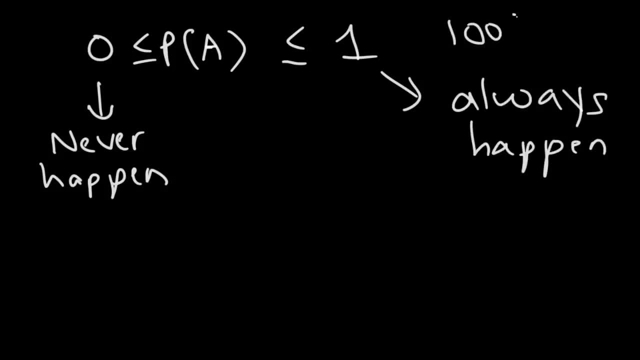 It also means that it has a 100% chance of occurring. If the probability of an event occurring is, let's say, 0.3, 0.3 times 100 is 30%. So it means that it has a 30%. 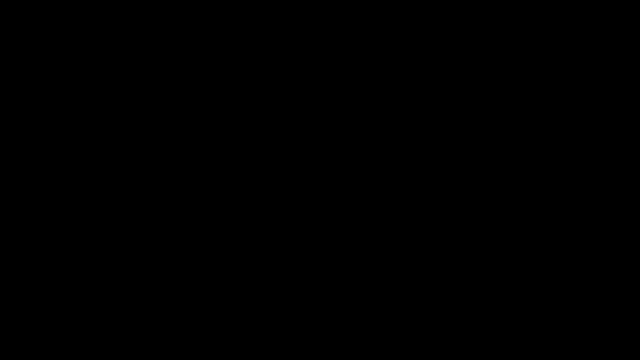 chance of occurring. So if the probability is 0.3, that means out of, let's say, 10 possible tries, we're going to get approximately three favorable outcomes, because three out of 10 is 0.3.. So let's say, out of 100 tries we would get 30 favorable outcomes. 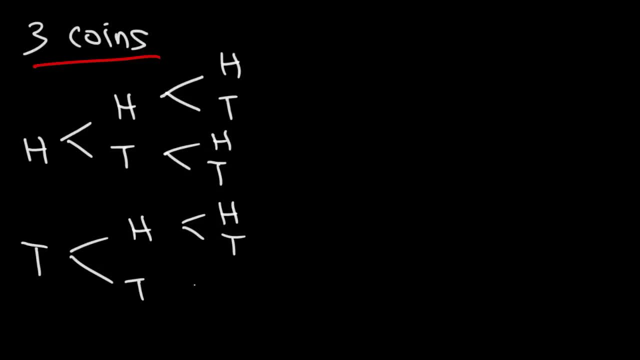 process For each one. So here's the first possibility: We can get three heads, So I'm going to write that as HHH. The second possibility is getting heads, heads and then tails, So HHH. The third possibility is heads, tails, heads, So that's HTH. The fourth: 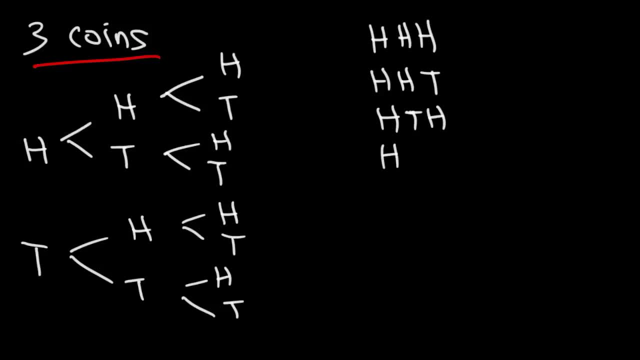 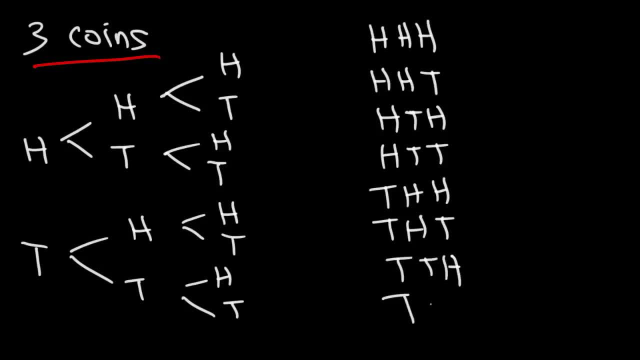 THT, THT, And the last one is going to be TTT. So we're flipping two coins three times. So the number of possible outcomes is 2, raised to the third power, which is two times two times two, so it gives us eight possible outcomes. 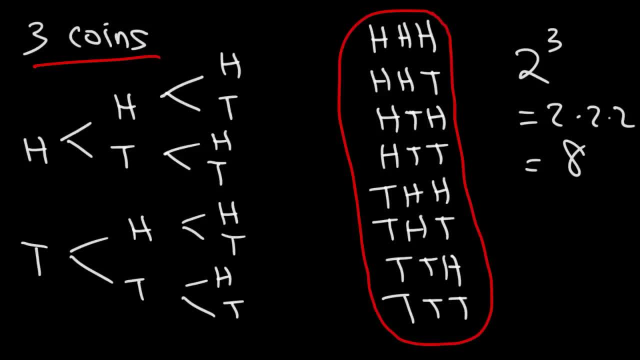 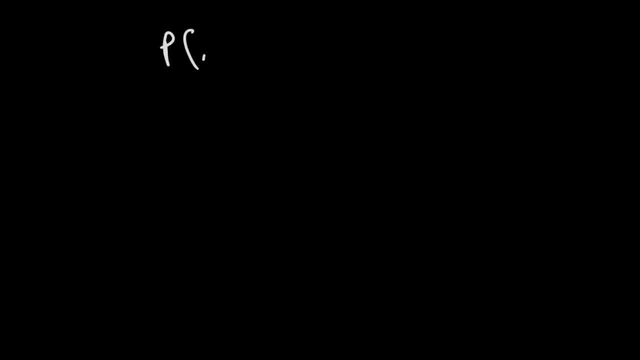 So this is the sample space, which represents all the possible outcomes that we can get for flipping three coins. Now, the probability of an event occurring is always between 0 and 1.. If the probability is 0, this means that this event cannot happen. It will never happen. Now, if the probability is equal to 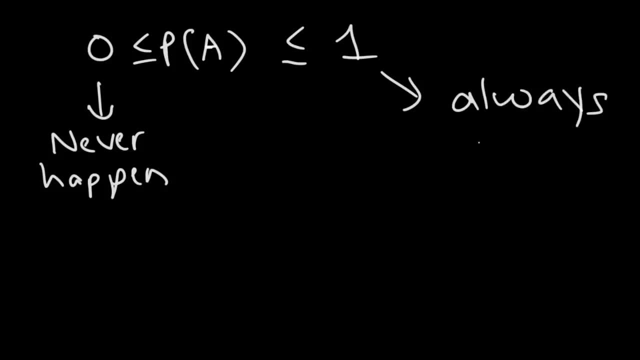 1,. that means that the event will always happen. It also means that it has a 100% chance of occurring If the probability of an event occurring is, let's say, 0.3, 0.3 times 100. 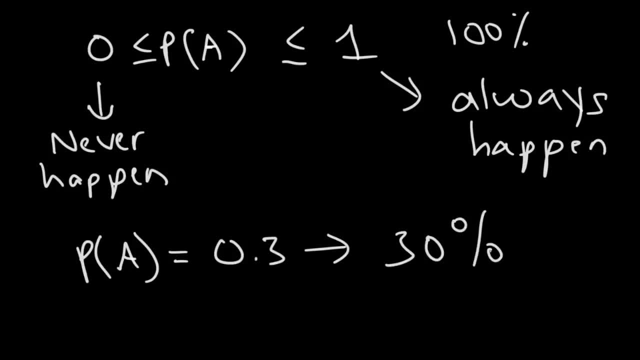 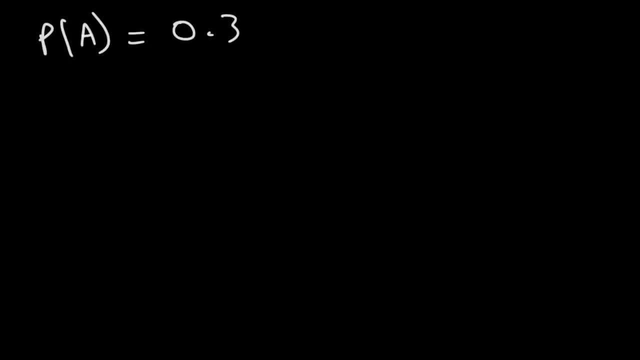 is 30%, It means that it has a 30% chance of occurring. If the probability is 0.3, that means out of, let's say, 10 possible tries, we're going to get approximately three favorable outcomes because 3 out of 10 is 0.3. 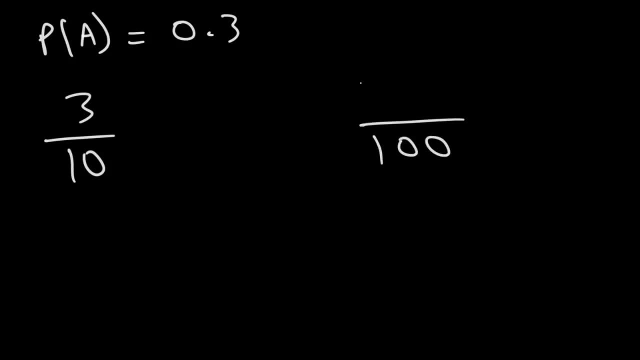 Let's say, out of 100 tries we would get 30 favorable outcomes. Here's an example situation. Let's say that the probability of people who drive a blue car is. let's say, if you have a certain population, a city, and if you randomly select a person, the probability of that person. 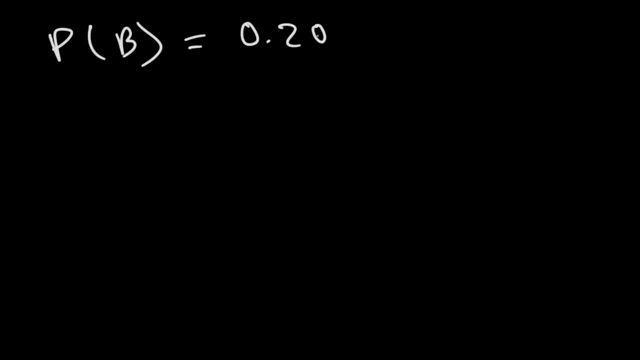 driving a blue car. Let's say it's 0.20.. That means that there's a 20% chance of selecting a person driving a blue car. If you were to randomly select 100 people, 20 people would drive a blue car. 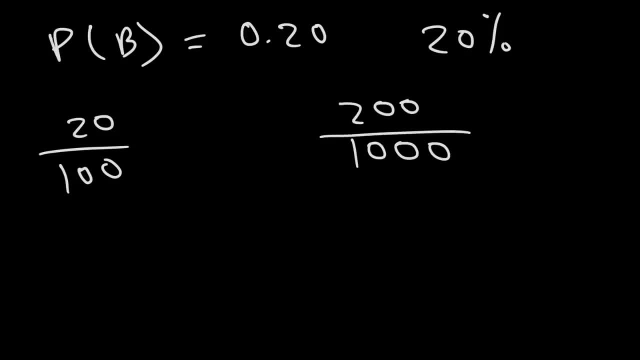 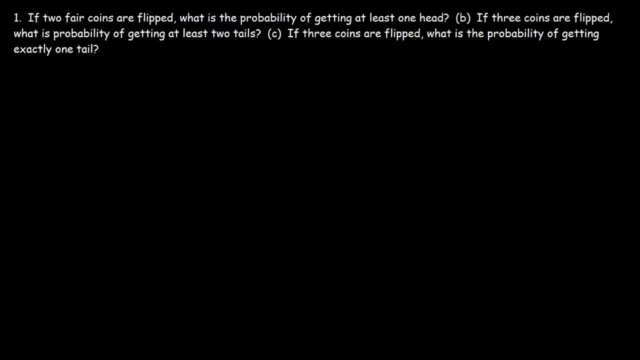 If you randomly select 1,000 people, approximately 200 will be driving a blue car. That's what probability tells you. Now let's work on some problems. If two fair coins are flipped, what is the probability of getting at least one head? 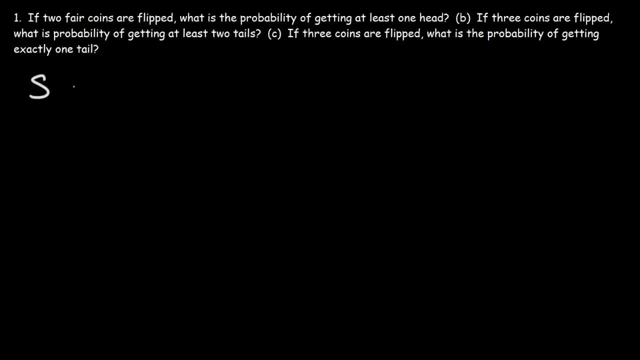 Well, let's begin by writing out the sample space for flipping two coins. So it could be heads, heads, heads, tails, tails, heads or T and T. Now the event A is getting at least one head, So this one has at least one H, this one too, and that one as well. 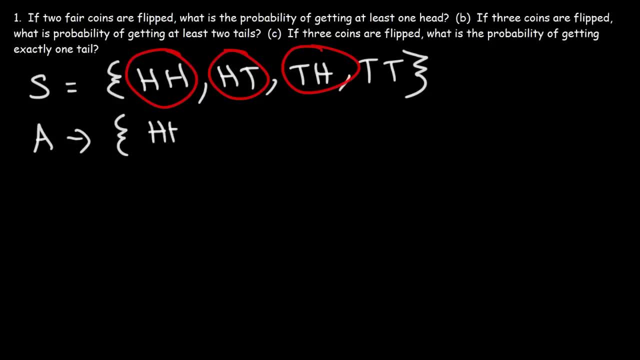 So the reduced sample space for A is H H, H, T and T H. So now let's calculate the probability In order for the event to occur. we have three favorable outcomes. The total possible outcomes are four. There's four events in the sample space. 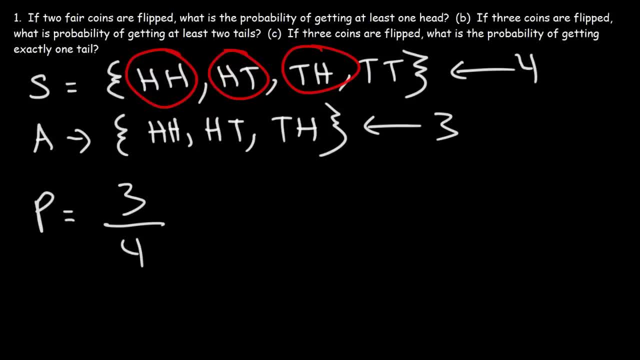 So the probability of getting at least one heads when flipping two fair coins is going to be three over four. Three divided by four is 0.75,, which means that there's a 75% chance for this event occurring. Now let's move on to part B. By the way, if you want to try it, feel free to pause the. 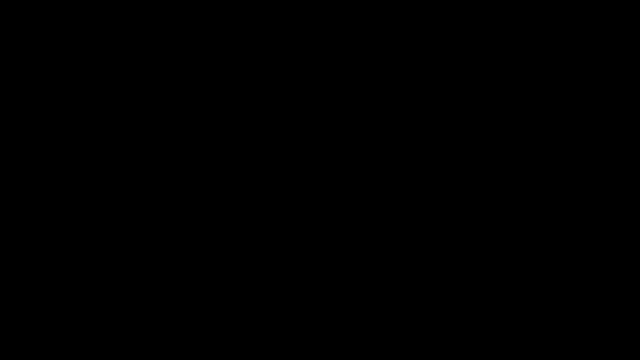 So here's an example situation. Let's say that the probability of people who drive a blue car is, let's say, if you have a certain population, a city, and if you randomly select a person, the probability of that person driving a blue car. 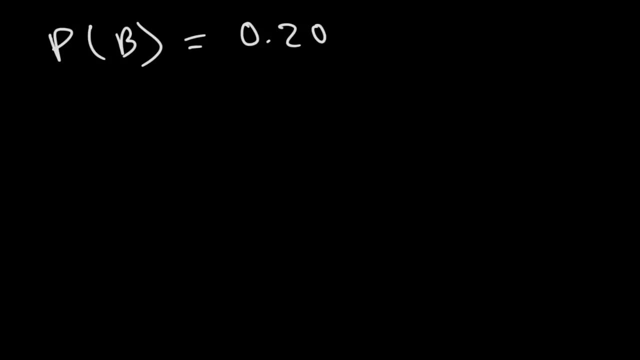 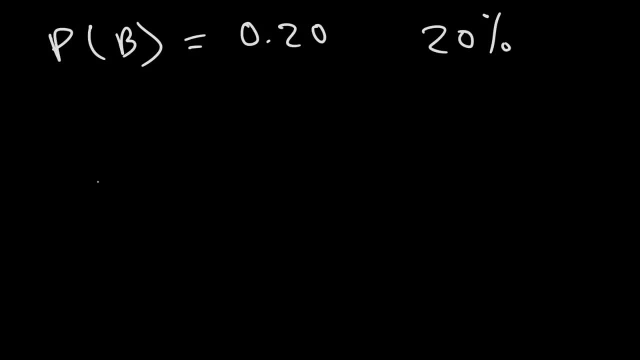 car. So if you were to randomly select 100 people, 20 people would drive a blue car. If you randomly select 1000 people, approximately 200 will be driving a blue car, And so that's what probability tells you. But now let's work on some problems. If two fair, 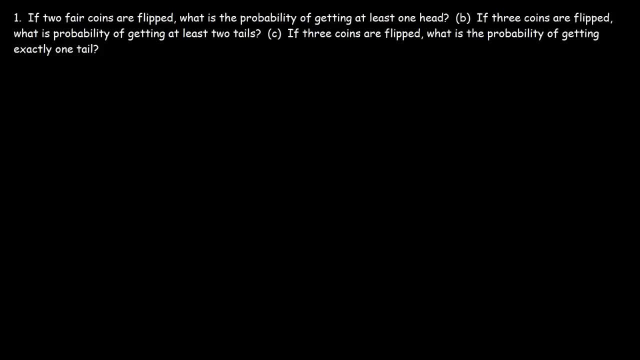 coins are flipped, what is the probability of getting at least one head? Well, let's begin by writing out the sample space for flipping two coins, So it could be heads, heads, heads, tails, tails, heads or TNT. Now the event A is getting at least one head. 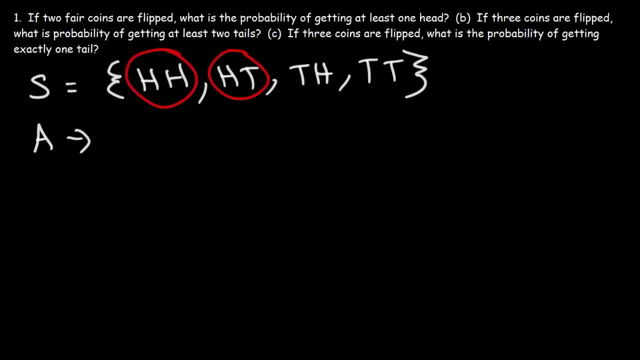 So this one has at least one H, this one too, and that one as well. So the reduced sample space for A is HH, HT and TH. So now let's calculate the probability In order for the event to occur. we have three favorable outcomes. The total possible outcomes are four. There's four events. 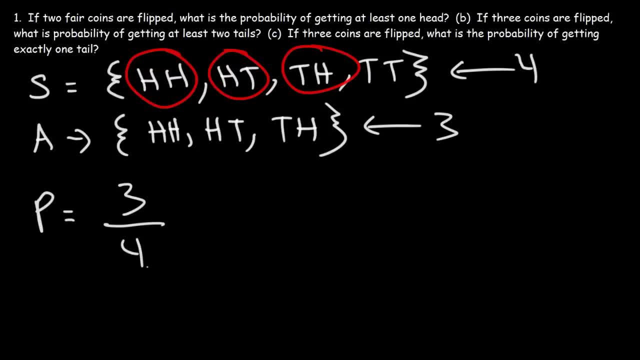 in the sample space. So the probability of getting at least one heads when flipping two fair coins is going to be three over four. Three divided by four is 0.75,, which means that there's a 75% chance for this event occurring. Now let's move on to part B. By the way, if you want to try it, feel free to pause. 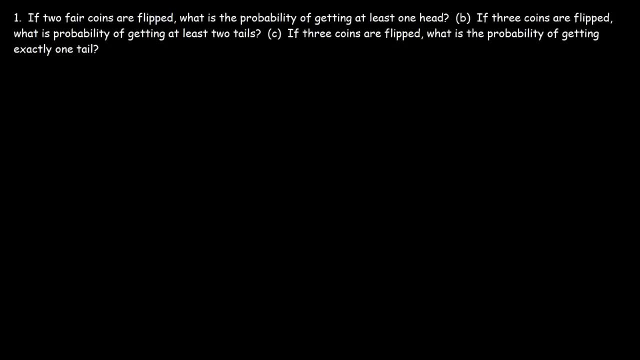 the video. If three coins are flipped, what is the probability of getting at least one head? What is? I forgot the word the. what is the probability of getting at least two tails? So let's begin by writing out the sample space. 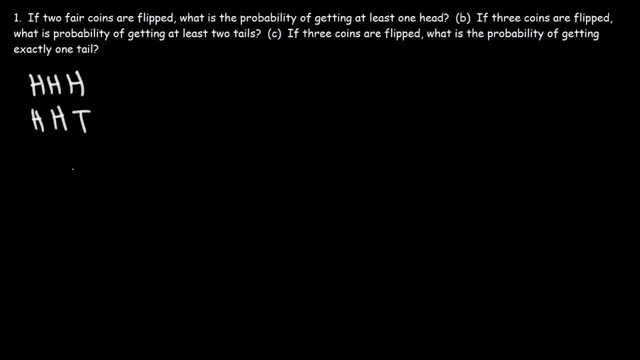 So let's write what we had before. It could be HHH, HHT, HTH, HTT, THH and so forth. So those are the eight possible events, that or outcomes that can occur in this event. So now let's call the event A. We want to get at least two tails. So which of these outcomes contains? 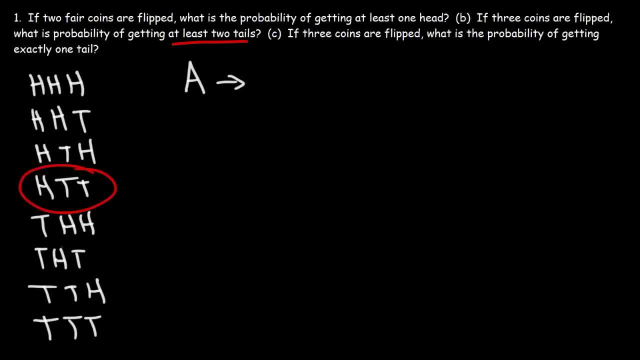 at least two tails. We have one, two, three, four, So there's four potential outcomes that have at least two tails. So let's come up to public health again and attribute their presentation. If B convinces, loves HH. otherwise, this is either A or B, HH, HTH, HTH or TH. If B convinces loves HH or B, HH, HTH or TH, Then this is definitely an average. They're probably hafta keep Da 생각 between these four equals, So'Swanna call something like that there. 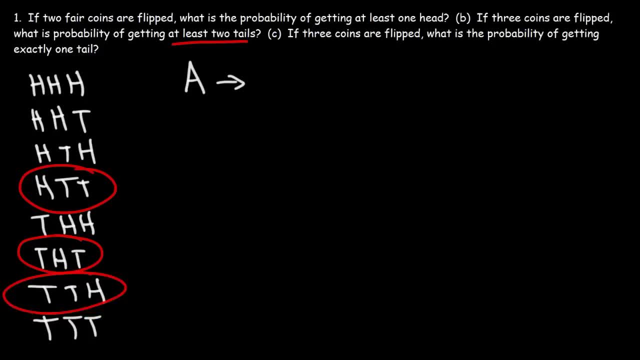 potential outcomes that have at least three tails. I mean, yeah, two tails. Kind of mix my words up there, So let's write it out. It could be HTT, THT, TTH or TTT, So the number of favorable. 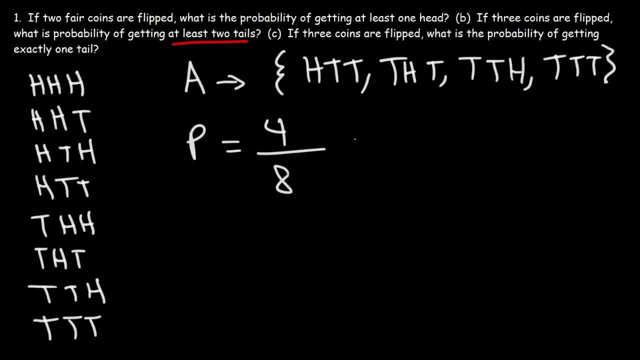 outcomes is four out of eight possible outcomes. So four over eight. you could reduce that to eight. Eight is basically four times two. Four is four times one, So this becomes one over two. One divided by two is 0.5.. So there's a 50% chance of getting at least two tails. 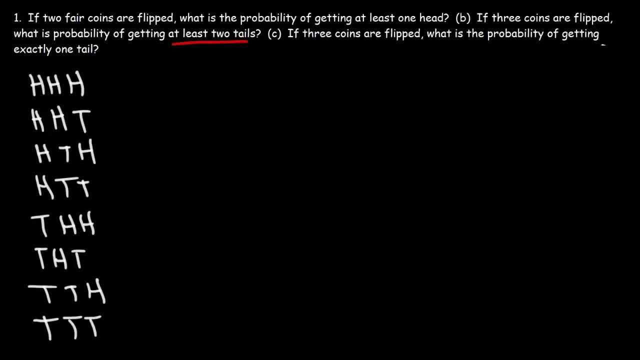 Now let's move on to part C. If three coins are flipped, one is going to get two tails. So if three coins are flipped, one is going to get two tails. So if three coins are flipped, one is going to get two tails. So if three coins are flipped, 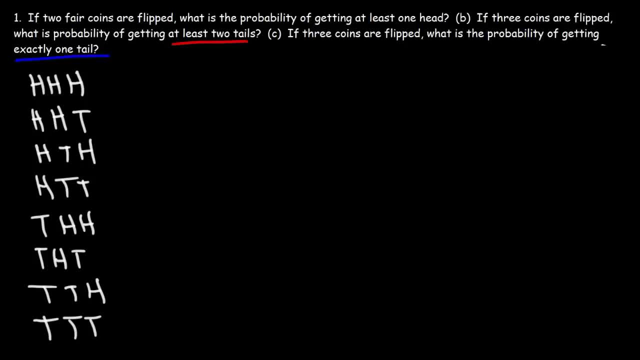 what is the probability of getting exactly one tail? So go ahead and take a minute and work on this example. Pause the video if you want to. So let's circle which outcomes, or let's circle the outcomes that contain exactly one tail. So this is one of them, Here's the other, This is another. 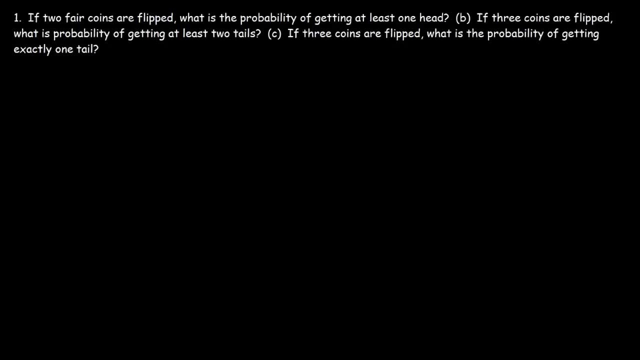 video: If three coins are flipped, what is the probability of getting at least one head? when flipping two fair coins- I forgot the word the- What is the probability of getting at least two tails? So let's begin by writing out the sample space. 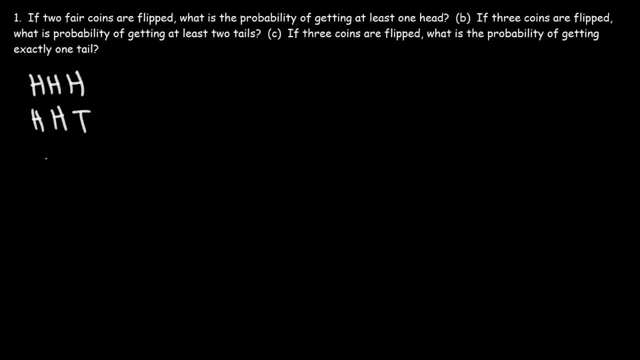 So let's write what we had before. It could be H, H, H, H, H, T, H, T, H, H, T T T H H, and so forth. So those are the eight possible events that, or outcomes that can occur in this event. 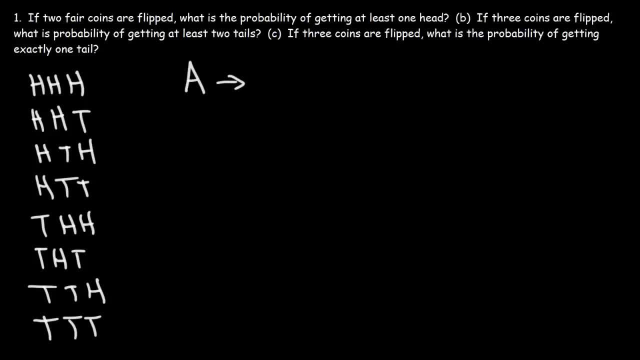 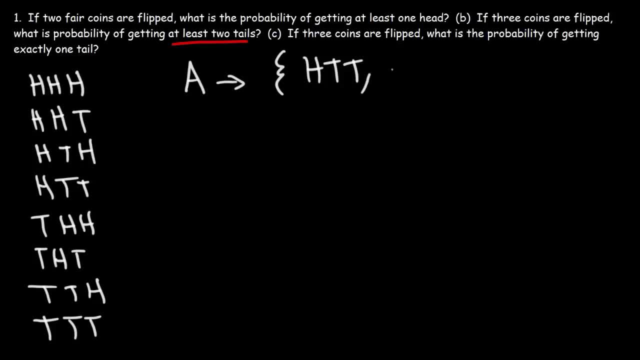 So let's write it out. It could be H T T T H, T T T H or T T T. So the number of favorable outcomes is four out of eight possible outcomes. So four over eight- you could reduce that to eight- is basically. 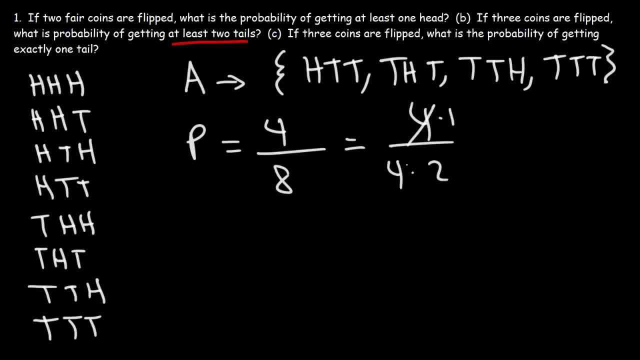 4 times 2.. 4 is 4 times 1.. So this becomes 1 over 2.. 1 divided by 2 is 0.5.. So there's a 50% chance of getting at least two tails. 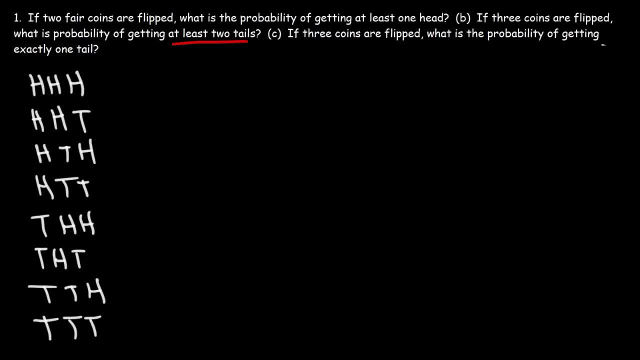 Now let's move on to part C. If three coins are flipped, what is the probability of getting exactly one tail? So go ahead and take a minute and work on this example. Pause the video if you want to. So let's circle which outcomes, or let's circle the outcomes. 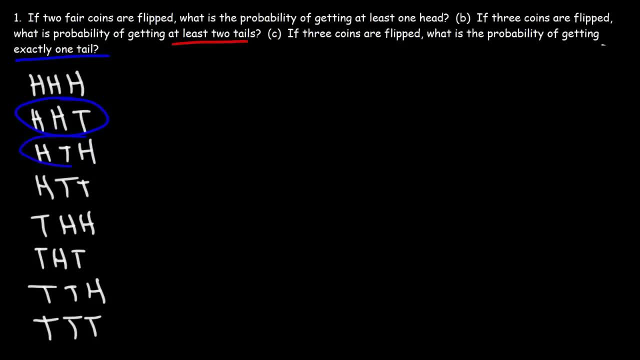 that contain exactly one tail. So this is one of them, Here's the other, This is another one, And that is it. So for event A, or let's call it event C. for part C, The three favorable outcomes are HHT, HTH and THH. 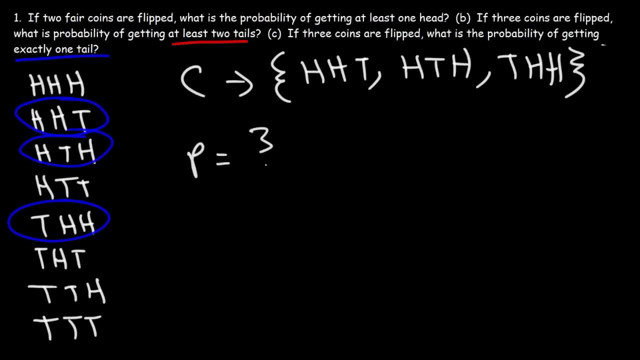 So the probability is going to be three favorable outcomes out of a total of eight possible outcomes. 3 divided by 8 as a decimal is 0.375.. And if we multiply that by 100, that means that there's a 37%. 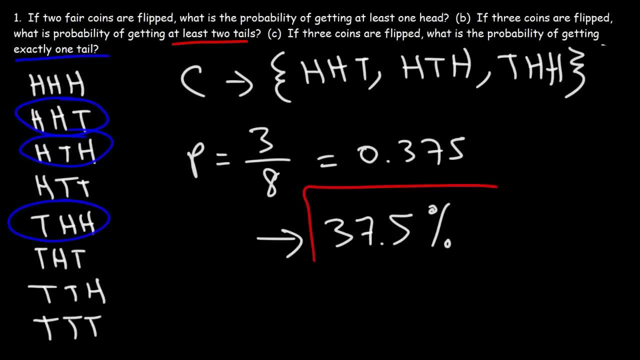 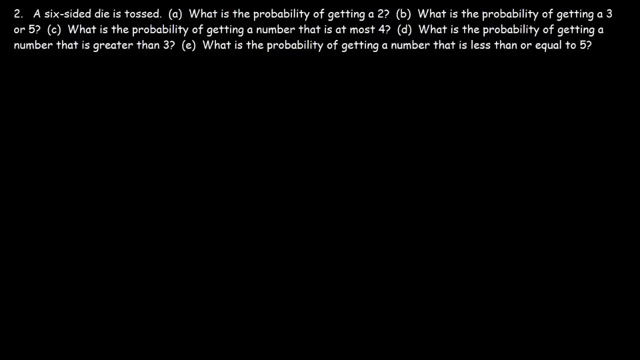 So the probability is going to be 7.5% chance of getting exactly one tail if three coins are flipped. So those are some simple examples of how you can calculate the probability of an event occurring. Now let's move on to our second problem. A six-sided die is tossed. What is the probability? 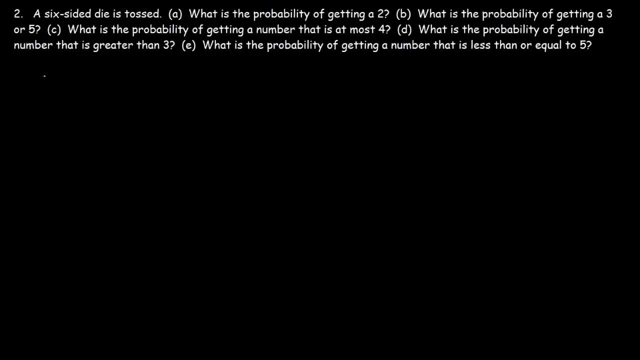 of getting A2?? Let's begin by listing the sample space. So here's all the possible numbers that we can get. It's basically 1 through 6.. Now the probability of getting A2 is just. there's only 1- 2 out of 6 possible outcomes. 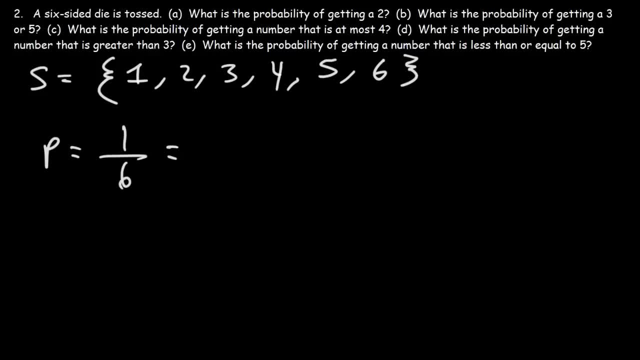 So we have one favorable outcome out of 6.. And 1 over 6 as a decimal is basically 0.16 repeated If we multiply that by 100.. But first let's round that to 0.16.. 0.167.. So this is approximately 16.7%. 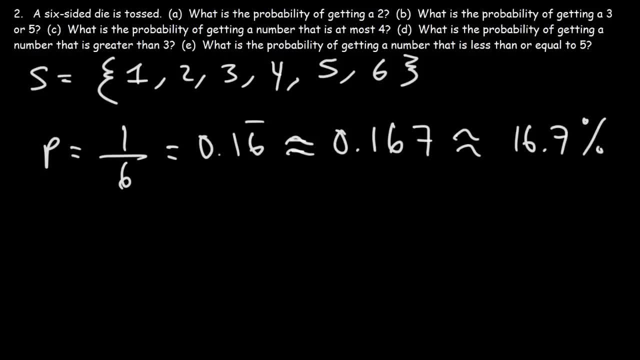 So that's the probability of getting A2 tossed in a six-sided die. Now what about part B? What is the probability of getting a 3 or a 5?? So we have two favorable outcomes out of 6.. So it's going to be 2 over 6.. 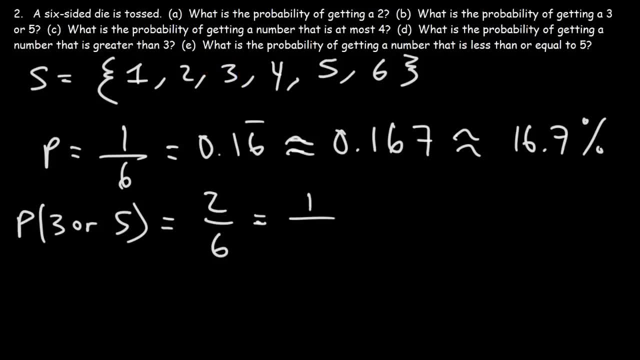 Which, if you divide both numbers by 2, you can reduce that to 1 over 3.. So this is basically 0.3 repeated. So that's a 33.3% chance of getting a 3 or a 5.. 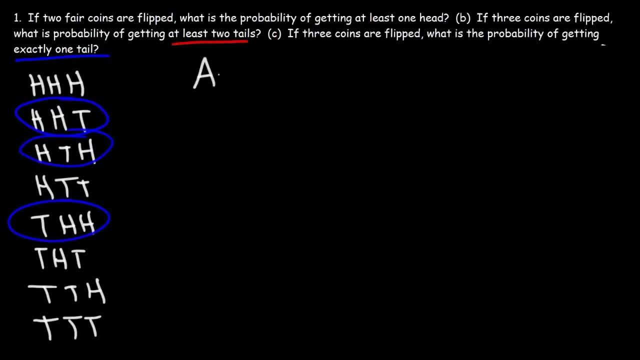 one, And that is it. So for event A, or let's call it event C. for part C, we're going to get. the three favorable outcomes are HHT, HTH and THH, So the probability is going to be three favorable outcomes out of a total of eight possible outcomes. 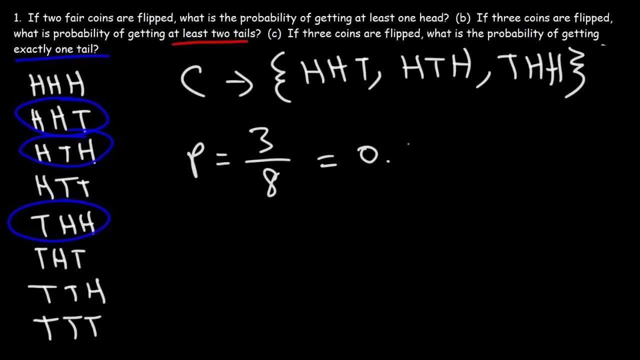 Three divided by eight as a decimal is 0.375.. And if we multiply that by 100, that means that there's a 37.5% chance of getting exactly one tail if three coins are flipped. So those are some simple examples of how you can calculate the probability of an event occurring. 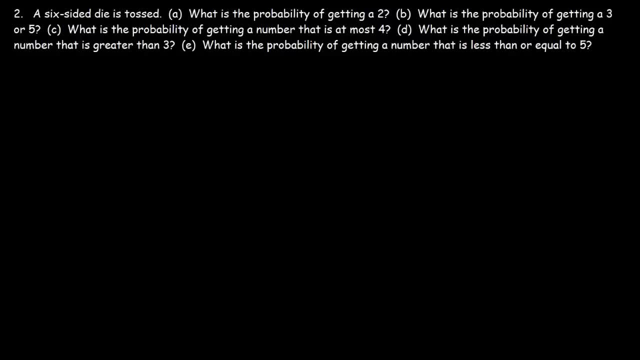 Now let's move on to our second problem. A six-sided die is tossed. What is the probability of getting a two? Let's begin by listing the sample space. So here's all the possible numbers that we can get. It's basically one through six. 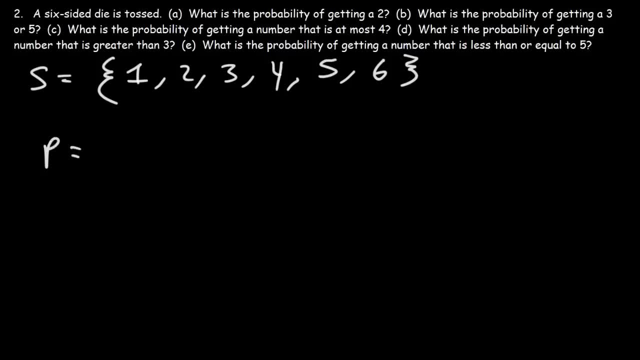 Now the probability of getting a two is just. there's only one two out of six possible outcomes. So we have one favorable outcome out of six And one over six. as a decimal is basically 0.16 repeated If we multiply that by 100, but first let's round that to 0.16. 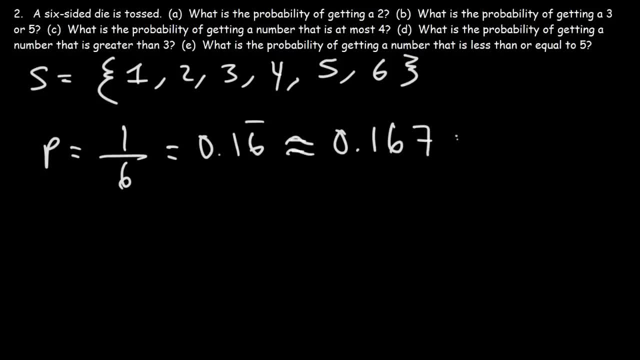 0.167.. So this is approximately 16.7%. So that's the probability of getting a two tossing a six-sided die. Now what about part B? What is the probability of getting a three or a five? So we have two favorable outcomes out of six, So it's going to be. 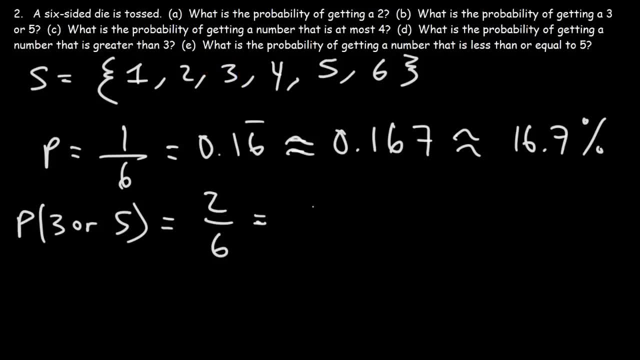 two over six, And then we have two favorable outcomes out of six. So it's going to be two over six, Which, if you divide both numbers by two, you can reduce that to one over three. So this is basically 0.3 repeated. So that's a 33.3% chance of getting a three or a five. 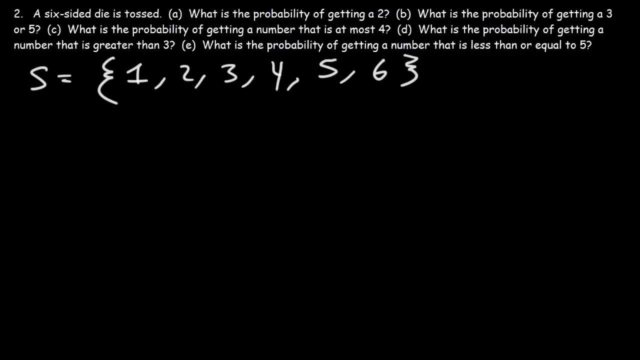 Now, what about part C? What is the probability of getting a number that is at most four? So let's make, let's list out the outcomes that leads us to this particular event. we'll call it Event C. So that is at most four. what does that mean? 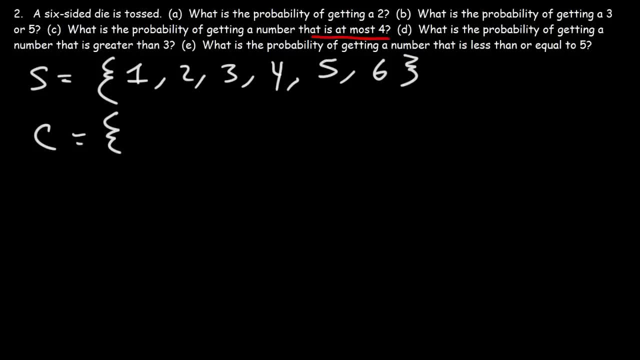 So that means we can get numbers that is less than or equal to four. So one, two, three, four. So the probability of this event occurring, we could say, let's say, if x is a variable, So x has to be less than or equal to 4.. 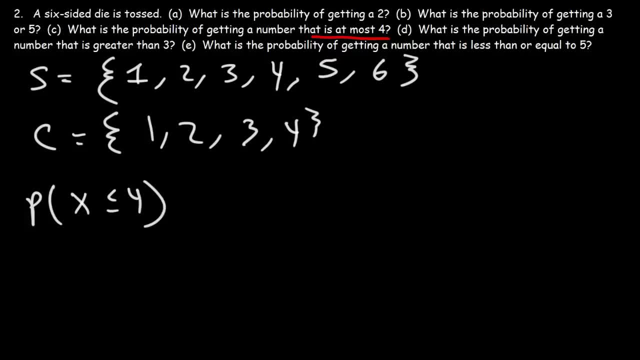 That means getting a number between 1 and 4, where x is an integer, Or technically let's say it's a natural number because integers can be negative. So there's 4 favorable outcomes over 6.. 4 is basically 2 times 2.. 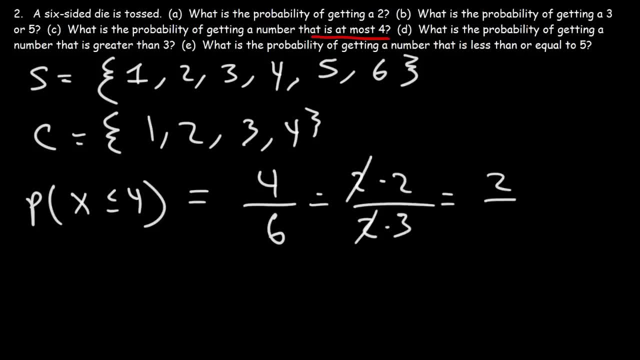 6 is 2 times 3.. So this becomes 2 over 3., Which is approximately 0.667.. So there's a 66.7% chance of event C occurring. Now what about D, part D? What is the probability of getting a number that is greater than 3?? 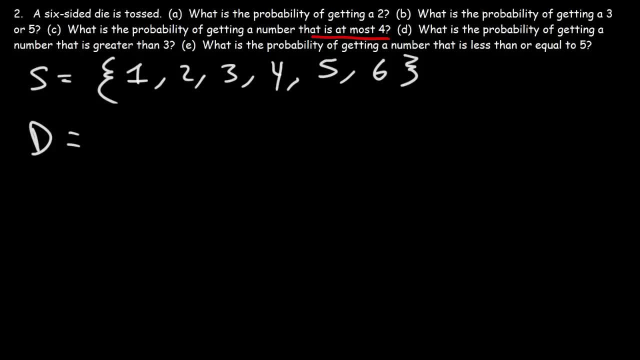 So let's list out the outcomes. that favors event D, So numbers that are greater than 3.. That includes 4,, 5, and 6.. But it doesn't include 3.. So the probability of getting a natural number that is not equal to 3, but greater than 3,. 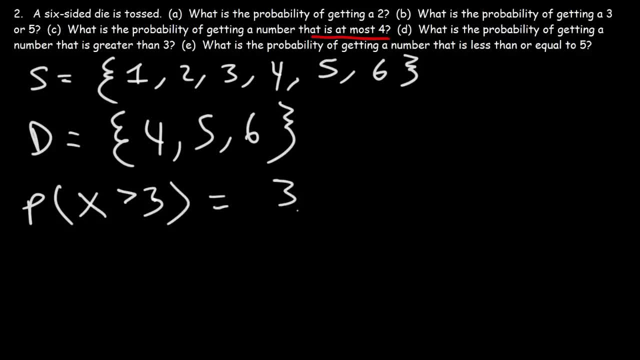 is going to be. we have 3 favorable outcomes out of 6.. 6 is 3 times 2.. 3 is 3 times 1.. So this becomes 3. 1 over 2. Which means we have a 0.5 chance or a 50% chance of event D occurring. 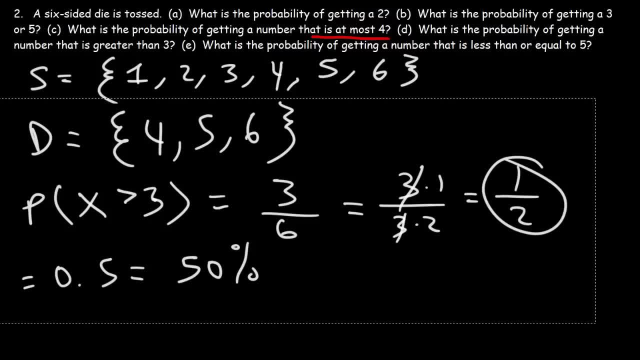 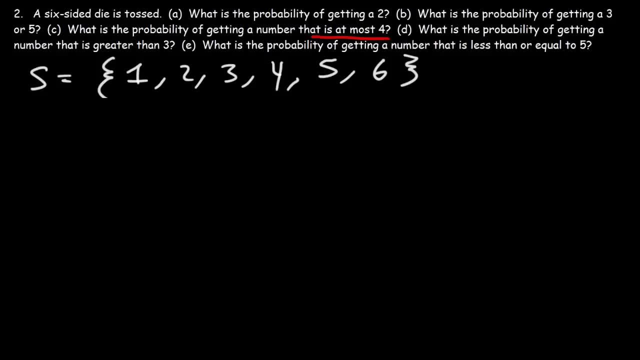 So, as you can see, it's not difficult to calculate the probability of an event occurring. It's pretty straightforward, but with many examples, you can see what to do. Now. what about the last part, part E? What is the probability of getting a number that is less than or equal to 5?? 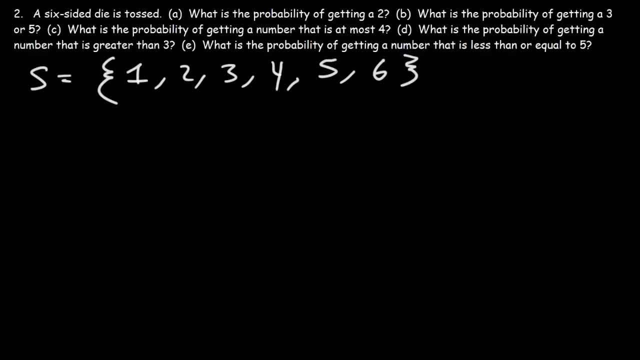 Now, what about part C? What is the probability of getting a number that is at most 4?? So let's make, let's list out the outcomes that leads us to this particular event. We'll call it event C, So that is at most 4.. What does that mean? 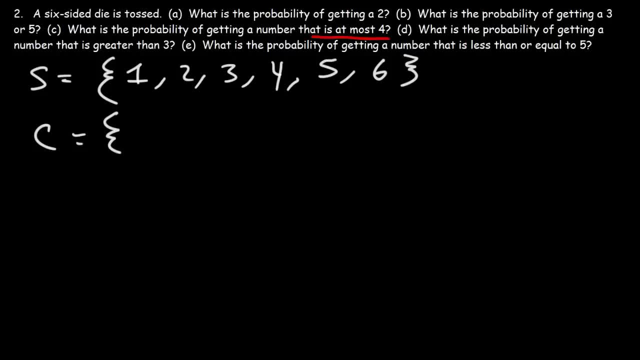 So that means we can get numbers that is less than or equal to 4.. So 1,, 2,, 3,, 4.. So the probability of this event occurring we could say, let's say, if X is less than or equal to 4, we can get a number that is less than or equal to 4.. 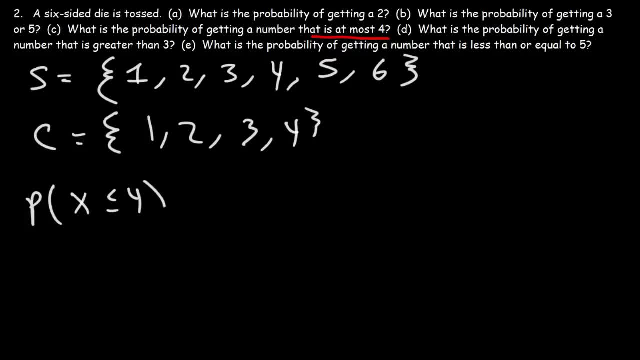 So X is a variable. So X has to be less than or equal to 4.. That means getting a number between 1 and 4, where X is an integer Or technically let's say it's a natural number, because integers can be negative. 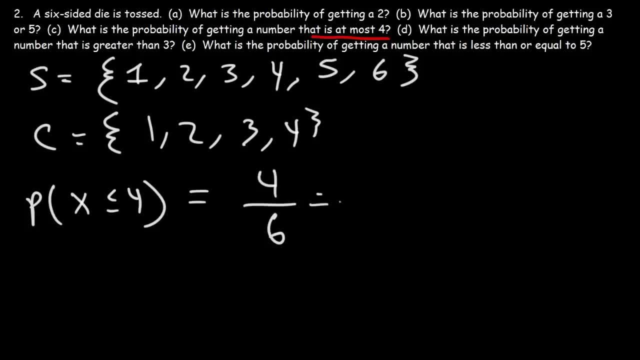 So there's 4 favorable outcomes over 6,. 4 is basically 2 times 2,, 6 is 2 times 3.. So this becomes 2 over 3. Which is approximately 0.667.. So there's a 66.7% chance of event C occurring. 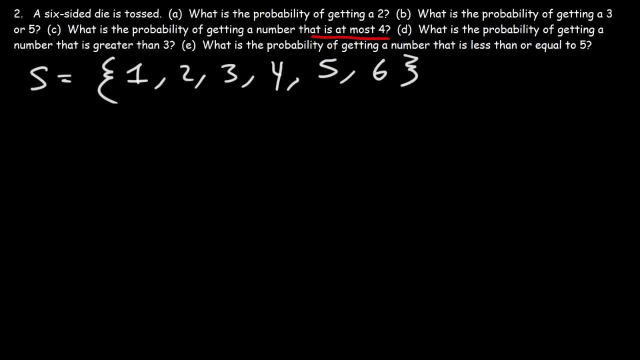 Now, what about D, part D? What is the probability of getting a number that is greater than 3?? So let's list out the outcomes. So the probability of getting a natural number that is not equal to 3, but greater than 3 is going to be. 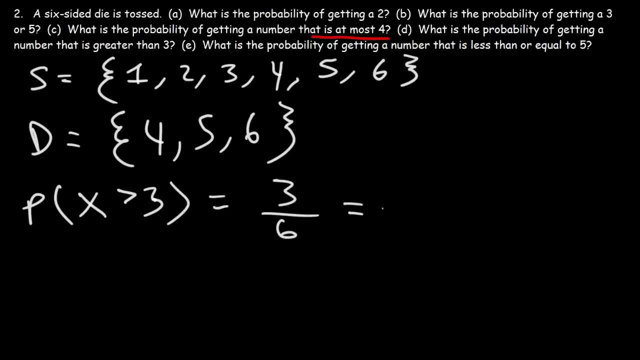 we have 3 favorable outcomes out of 6.. 6 is 3 times 2.. 3 is 3 times 1.. So this becomes 1 over 2. Which means we have a 0.5 chance or a 50% chance of event D occurring. 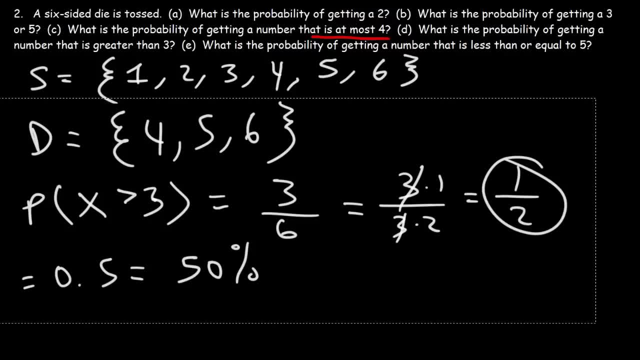 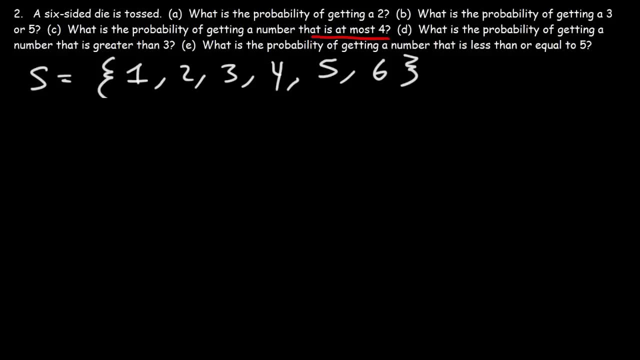 So, as you can see, it's not difficult to calculate the probability of an event occurring. It's pretty straightforward, but with many examples, you can see what to do. Now. what about the last part, part E? What is the probability of getting a number that is less than or equal?